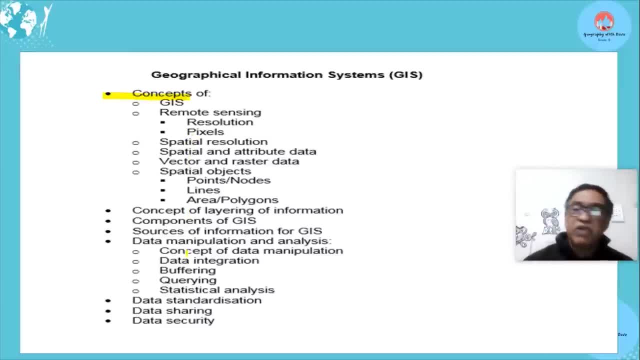 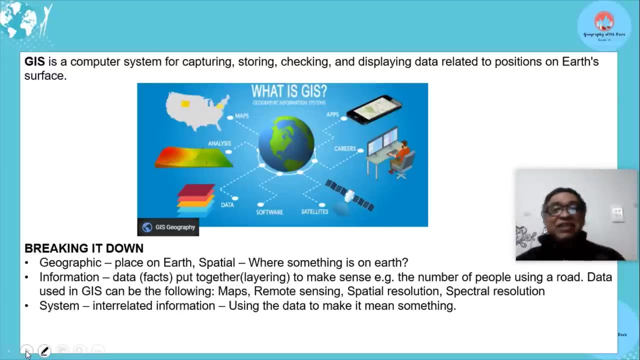 them in each slide. Many of these concepts you've done already all right, with a few like data standardization, etc. that is maybe new from a tick, but we will simplify. In fact, if I go forward, I will find that the longest definition is and the more complex definition is GIS itself. Okay, 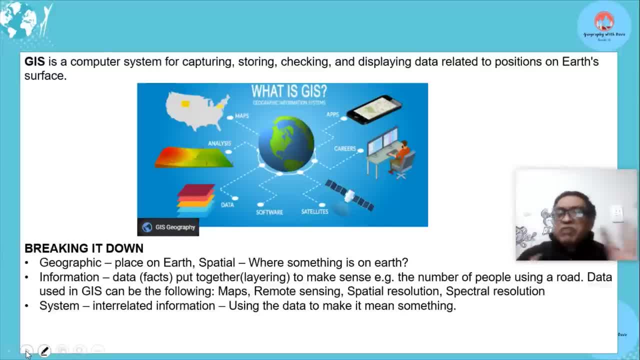 that is your very, very, I would say not even complex, but most complex that we have from the others, and it's fairly simple. So let's look at- we do need to look at- what is GIS. Of course we know it's a computer system. all right, That's what you use. you use programs. 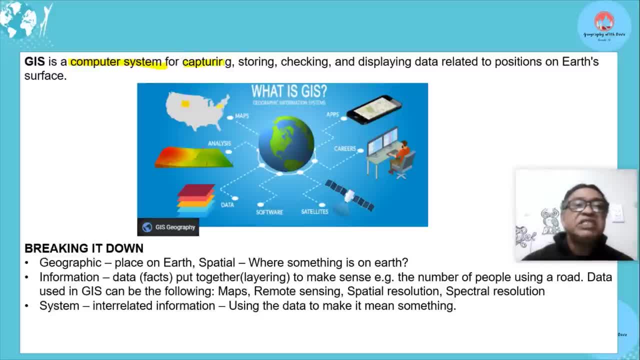 you use a computer system which captures, stores, checks and displays data related to positions on the Earth's surface. So when we look at this, we know we have to use a computer for this. We know it captures data, all right. When we do it from remote sensing, we capture data or we capture. 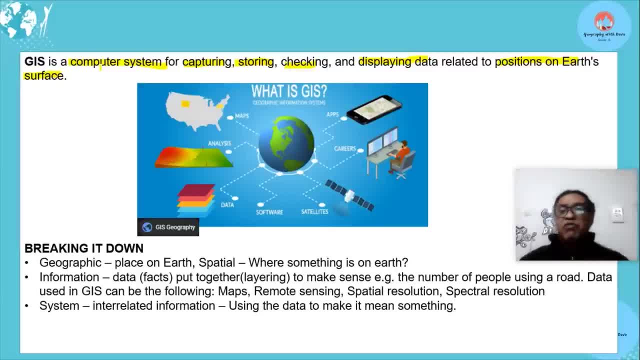 data from any other data source- Example number of people or the crime rates in different areas. you can get it from statistics. So you can store the data, you can check it, you can display it and add it up, like data layering. you learned, You understand, you want to look at where's the best. 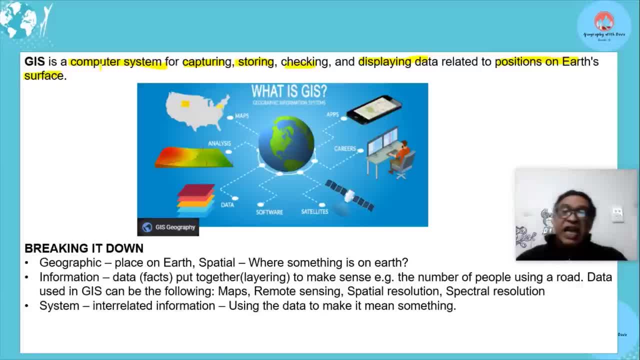 place to put your farm. You get a data layer of fertile land, you download it, you use your computer, Then you get a data layer of flat land and you get that data also. And then you get a data, a data on water supply, and you put all the data together and you will find that hey. 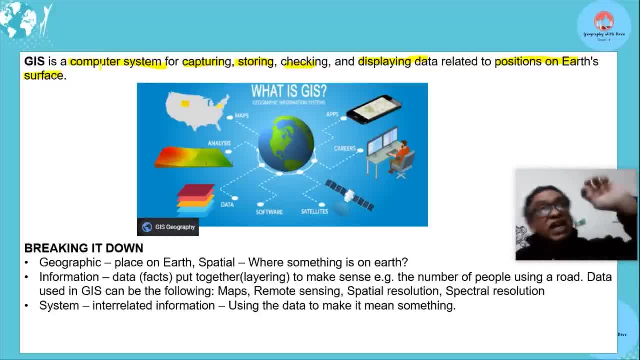 I must farm there or there because it's the most fertile land, the flat land, et cetera. Okay, so it's doing all that And, as you can see here, all this information coming into computers with its careers apps, maps, analysis software, all is used in data, So this is a fairly good and 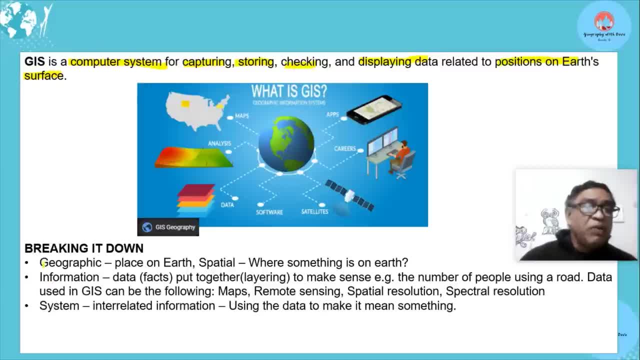 comprehensive definition of GIS. So when we look at GIS, we look at geographic. That's how we got it. Geographic information systems: That's what it means. A place on earth, spatial, where something is on earth. You got it. learners. 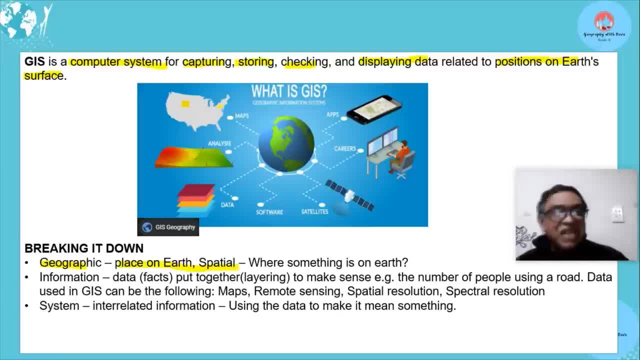 All right. So we have to look at spatial first, the location, et cetera. Okay, Information, That's geography, information systems. This is data or facts put together. You can layer them one on top of the other to make a topographic map. 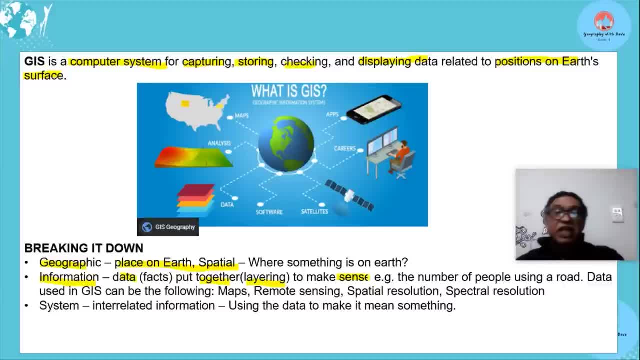 make sense. Okay, When we put things together, All right, Where I spoke about where you're going to farm, You understand makes information more useful. Example: the number of schools using a road for congestion. All right, Data is used in GIS can be. can be used in the following: We can: 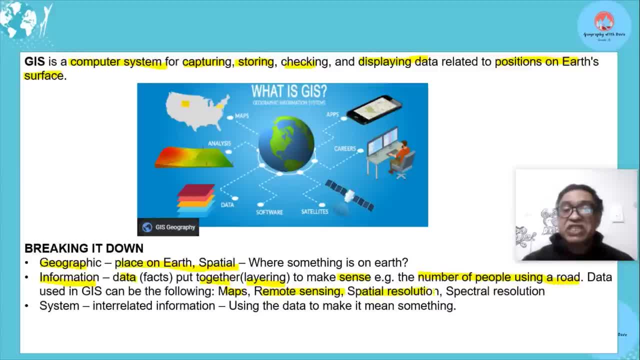 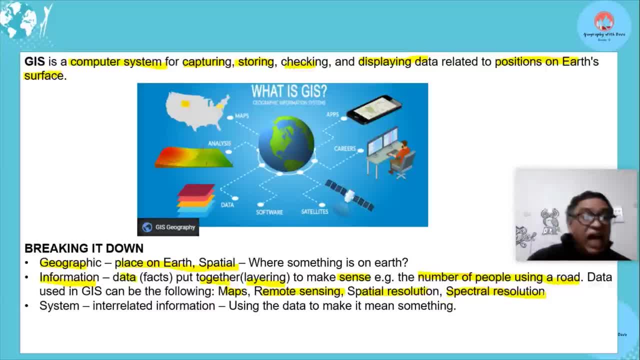 like, for instance, road networks, et cetera. And the last thing is system Interrelated, interrelated information, using data to make it mean something. All right, That's a system that will put it together now. Okay, You've got data. As I said, 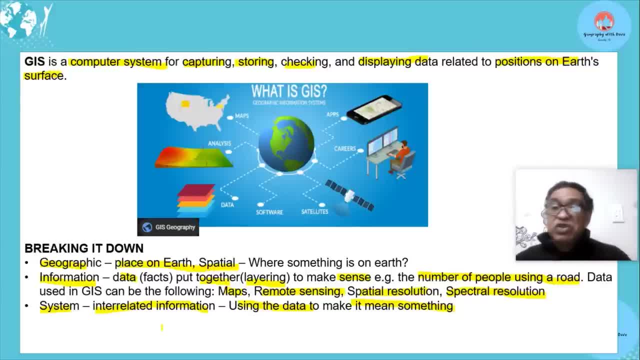 let's go back to the example. you got data- fertile soil- you can. you just use that data to then say: i'm going to farm there. you also need other data- flat land, water supply, transport- and all of a sudden, if you interrelate that data and put it together, it becomes more useful. it means something. hey, that's a better. 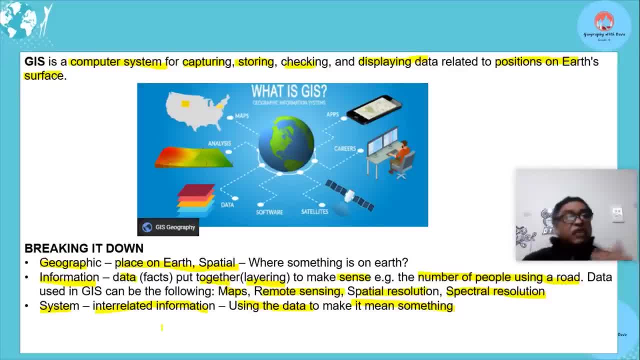 area to farm, a better area to put in my factory. so this is what it is: geography, geographic, spatial information is data and systems that put the information together. all right, that's the simplest way that i could put in this gis concept, so you can see it in the top here: computer system. 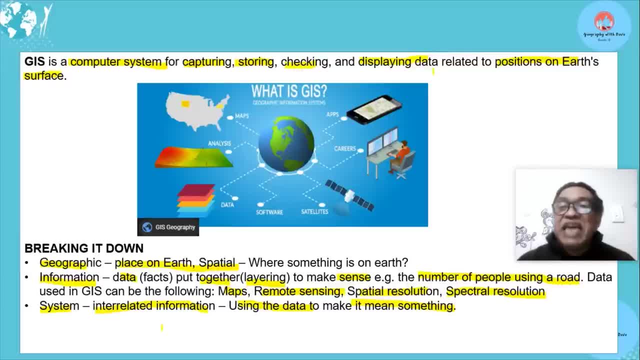 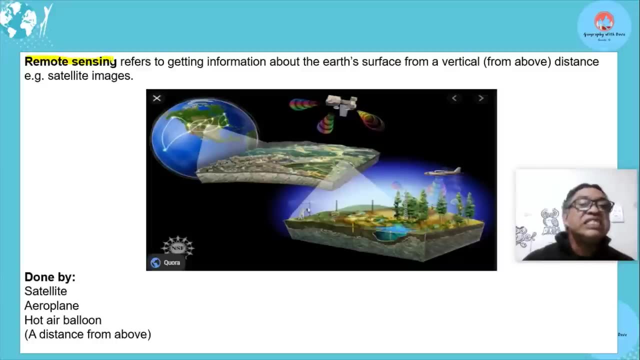 capturing, storing, checking, displaying the data related to the earth's surface. all right, and this is how we do it. okay, so general definition. now let's get to the other concepts. remote sensing: you can see the satellite here. you can see the aeroplane here. it's taking images of the 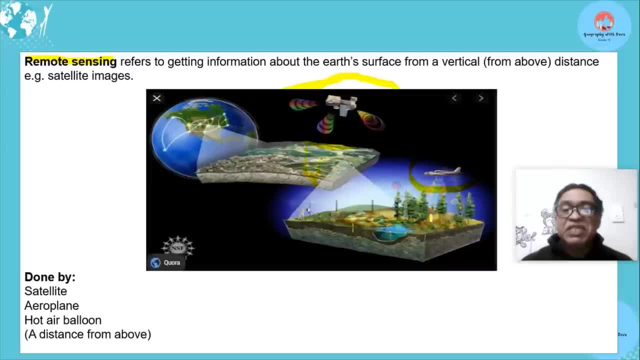 earth. okay, can you see taking images of the earth from a distance? now watch out, learners. this definition is updated. now we say getting information about the earth's surface from a vertical distance. all right, this has changed from a vertical distance or from above. so please note, learners, you must be specific on that. most things now tell you it's just a distance, so that has. 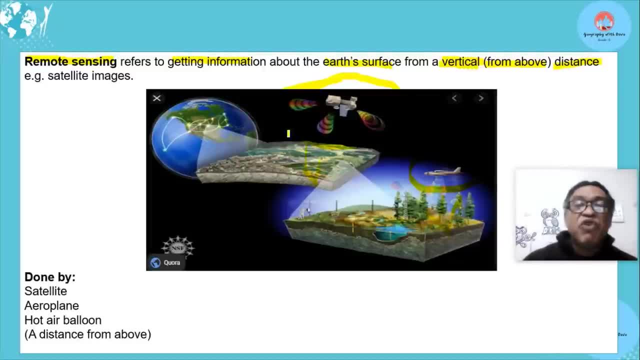 changed. now. many of us just focus on this. watch out, learners. if you say it is getting information of the from about the earth's surface- uh, from a vertical distance, from a satellite- then you give me an example. you must say vertical distance above if you want to. 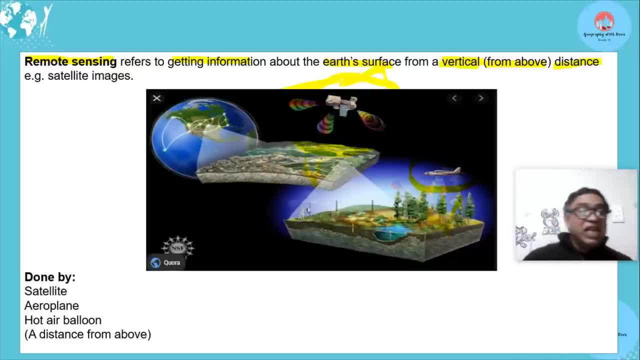 give an example, then it's satellite, because not only satellites can take images. there's other examples: aeroplane, hot air balloon. all these things take images of the earth all right, from a vertical distance. so anything that takes from a vertical distance can be considered remote sensing. 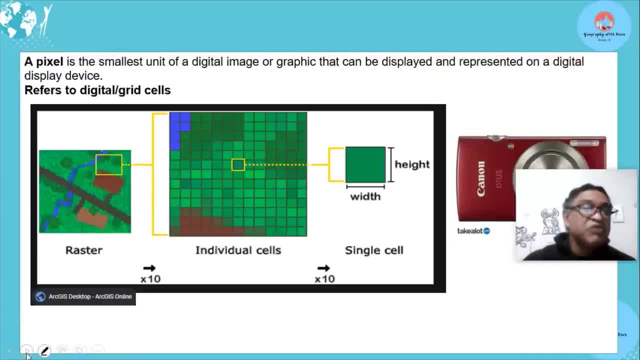 okay, so we've got that concept. let's move to the next one: a pixel. a pixel, all right. now. what is a pixel? it's the smallest unit of digital image or graphic that can be displayed or represented as a digital display device. okay, so it's a small. 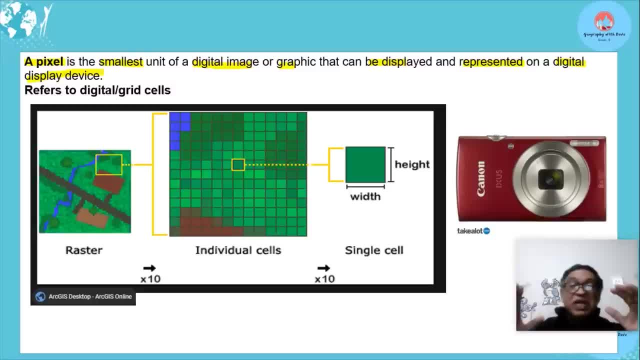 pixel. it's the smallest each one of those pixels make together make the picture okay. so the more the pixels, all right, the clearer and the clarity and the quality in terms of clarity the images are better. okay. so if you say learners, it refers to digital grid cells, we'll accept it. all right, i. 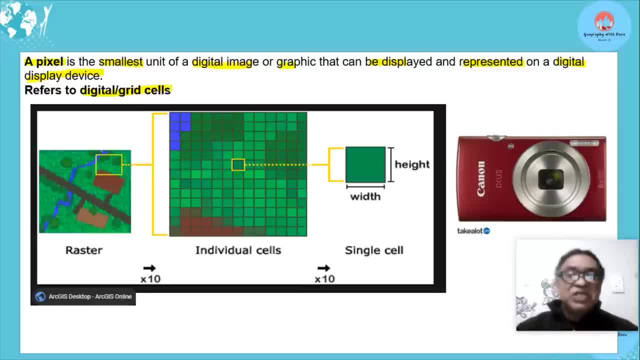 gave you the full definition, but i'm showing you how it can be simplified. so this in a picture is a pixel. can you see here this? now all these little pixels come together and they make a picture. all right, and it has to be. it's an image, so it has to be. 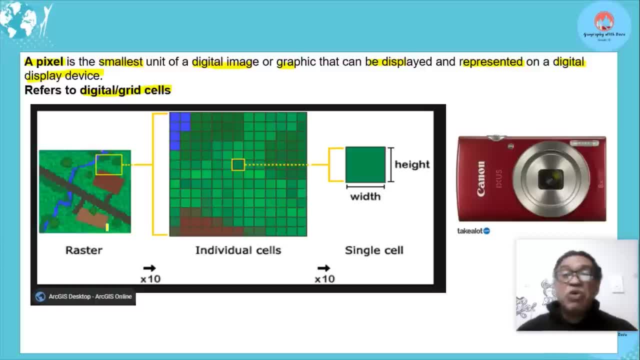 your raster data, working with images, photographs, and that is why some people boast: whoa, my camera is a 16 pixel and each year it went up it's a 32 pixel. okay, megapixel, all right, meaning that each takes clearer pictures. okay, so you must have. 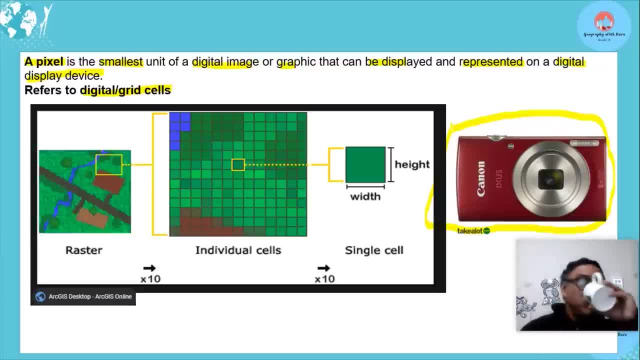 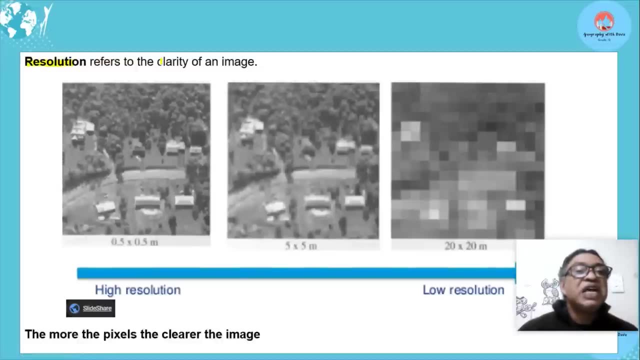 heard that before. my camera has got so many pixels in it. okay, so the clearer the image if there are more pixels. all right, now let's go further. resolution refers to the clarity of the image. let's look at these ones. this is: pixels are very big and there's not much, so it's not very clear. let's go down. 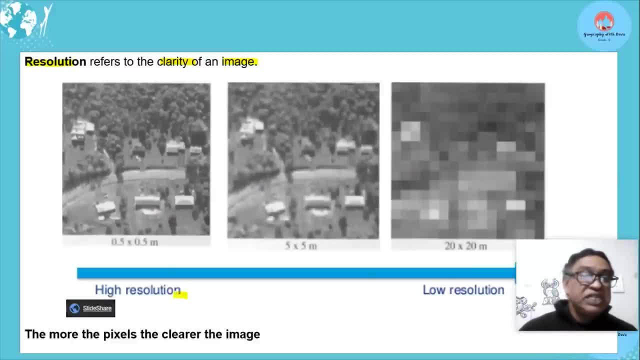 where it is smaller, so the resolution is higher. in this one, therefore, you can see the picture is far more clearer than this picture because it has a higher resolution. please note- i know sometimes i see this question which has a higher resolution: the topographic map or the auto photo. the topographic map does not have a resolution. all right, it's not. 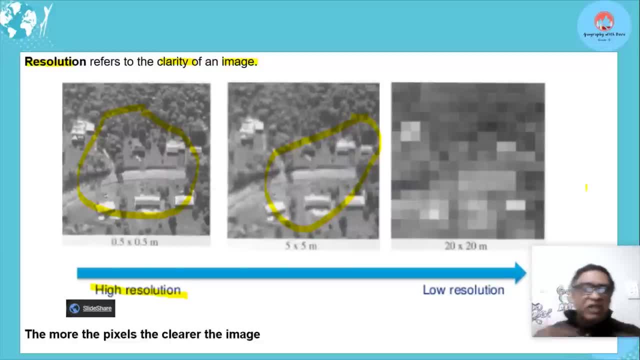 an image. it's made all right with points, lines and polygons, okay, so the image makes the determines the pixels all right. so the more the pixels, the clearer the image. this is what we picked up, but just now it's refers to the clarity of image. that is, there are some long definitions. this is 5. 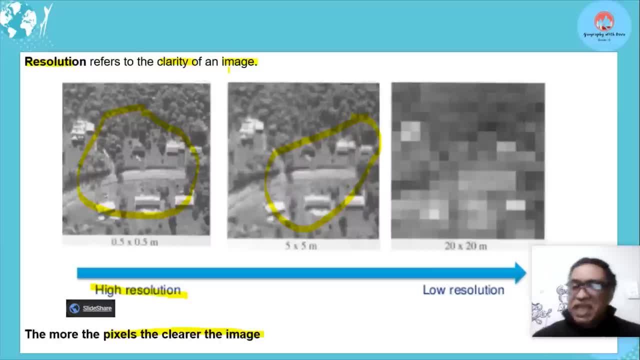 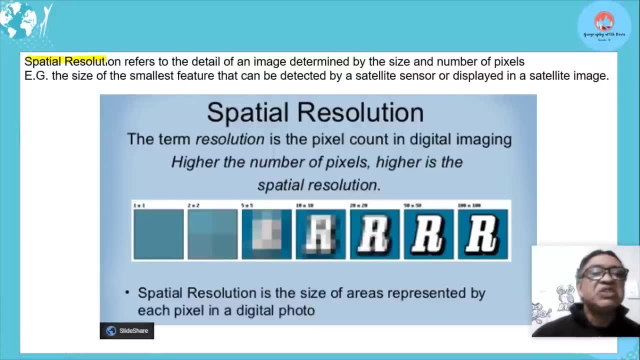 okay, and the clearer. the more the pixels, the clearer the image. okay, let's look another one. spatial resolution, all right, refers to the detail of an image determined by the size and number of pixels. all right, okay, the detail. you can see more detail. you look at this. 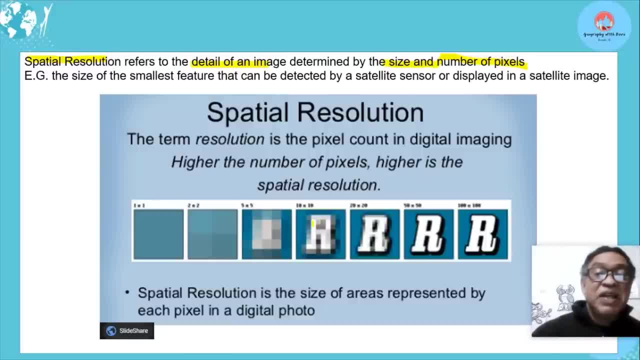 all right, less pixels. okay, you see it, but you don't see the full detail. yeah, you'll see a better detail how it bends. you can't see all that yet, am I? can you see the real bending of it here? that little piece here, but as the pixels? 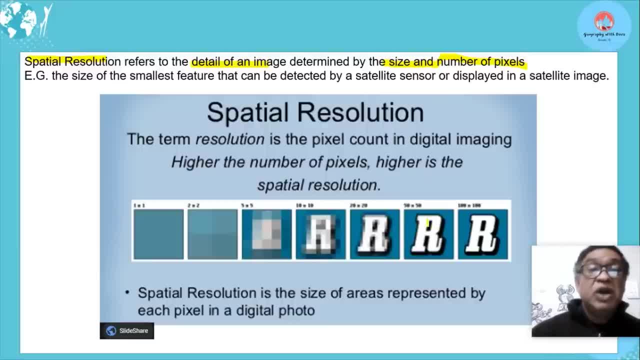 improve and L, as the spatial resolution improves more detail. so it's not just about clarity, it's about detail. okay, so I can see something about clear, but constitute a detail that's shown in this case. can you see it? all right, there's a little more detail from you had today. all right, you can see, even you can see. 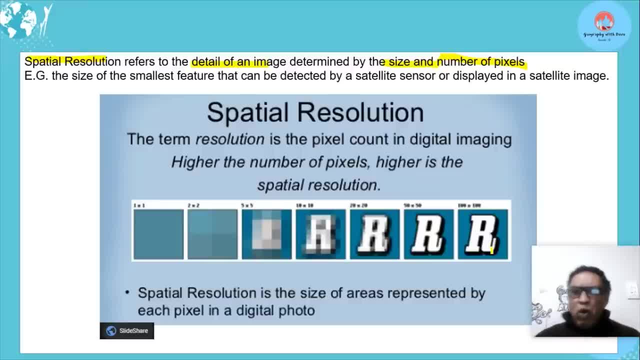 the lot bend. you know. that is why we see people go and by you guys more than me. I'm just a poor teacher. you buy this television, which is you HD and I don't know, it's a ID whatever- and you see, oh, I can see the wrinkles around the person's eyes. 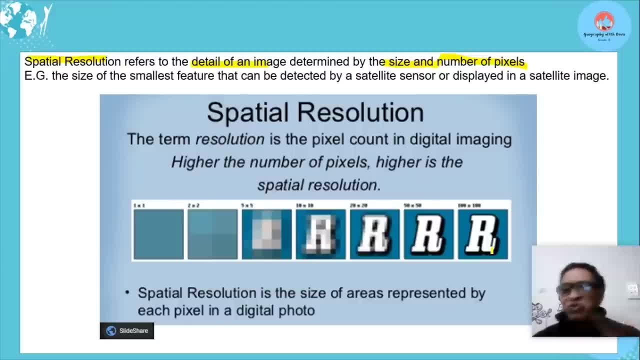 brilliant, high spatial resolution. okay, that gives you a better idea about this. okay, now these examples I'm just giving you. all right, the definition is this: detail of an image determined by the size and number of pixels. but even if you know detail of an image, all right, if they give you as a sort of, it is still. 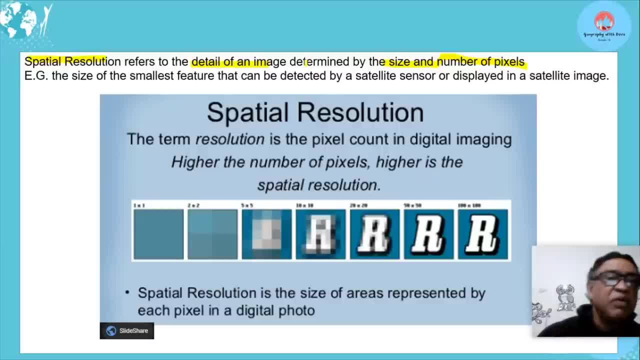 fine. I would still prefer saying determined by the size and number of pixels. like example, the size of a smallest feature can be detected by satellite sensor and displayed as a satellite image. it can even smallest of features. you know. you can see a dot on taking, doing remote sensing etc. we pick. 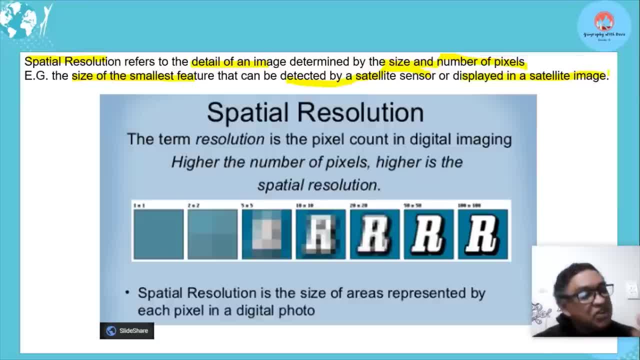 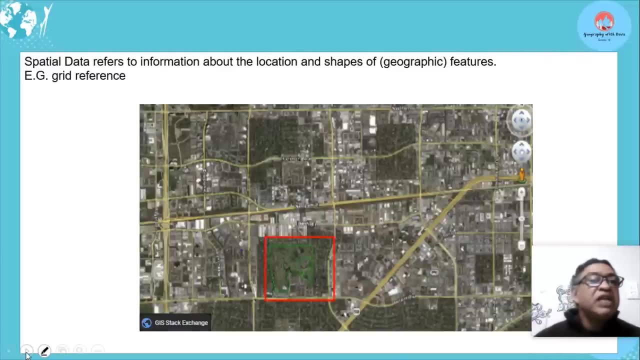 up that satellite sensor and as you zoom down, you can get right into that. it's a person that's lying down the eyes. whatever you can actually see, brilliant, all right. the next one that we look at is spatial data. it refers to information about the location and shapes of features. okay, example, your great reference, that is. 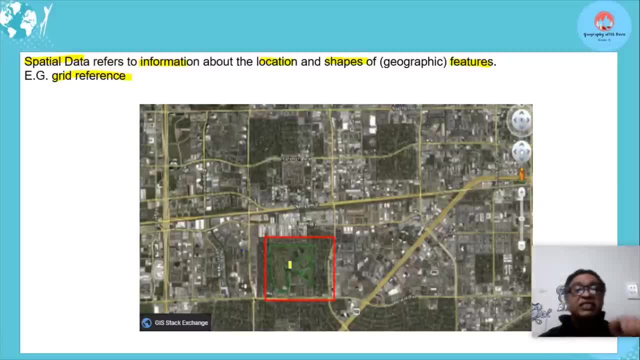 spatial data. we want to know exactly where something is located: 25 degrees- 15 minutes, 30 seconds south. 24 degrees, 18 minutes, 16 seconds, east. that is location. that is spatial data. also, you can see the shape of this. okay, so if I had a good year and a special, I had my seconds. 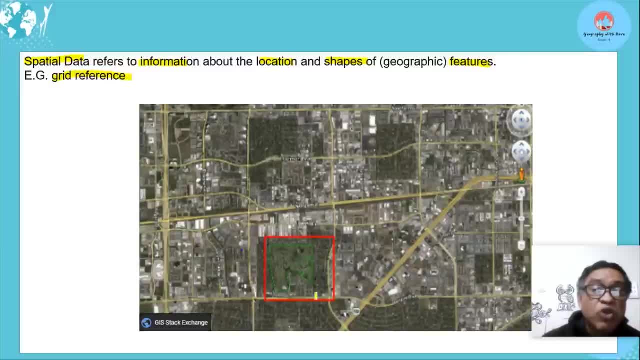 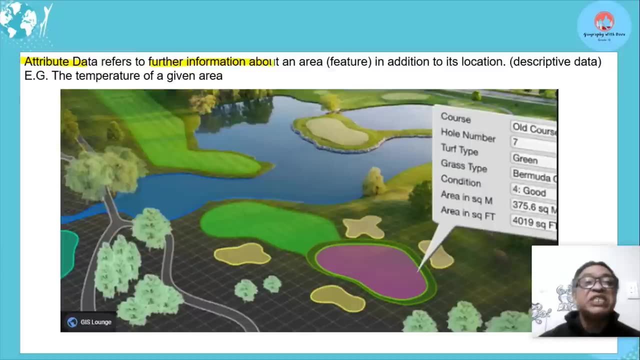 and minutes. I would know exactly where it's located and I would also pick up the shape of it. so spatial location GIS. okay, let's go further. attribute data now. this is further information about the area or feature in addition to its location. so it's descriptive data and you can make. 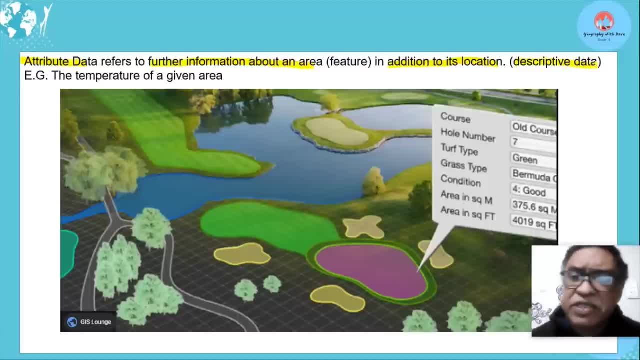 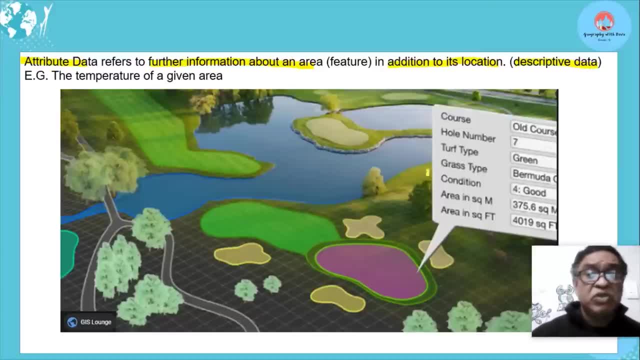 course I know where this to golf course is located. I can work out the grid reference if I have the information- topographic map, whatever. now on attribute data, further descriptive data about this place. example, I stated the temperature. if I've got a temperature map, it can give me. what else can I see on this? 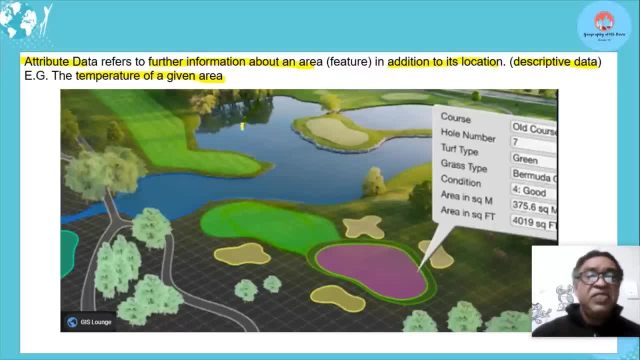 photograph. it has a lot of green grass. they are ponds or lakes. they are bunkers. can you see it? alright? how many holes are there? I know there's eighteen holes in a golf course. there are trees on this golf course. can you see that? it is describing the goal court, so the golf course is located at so many degrees. 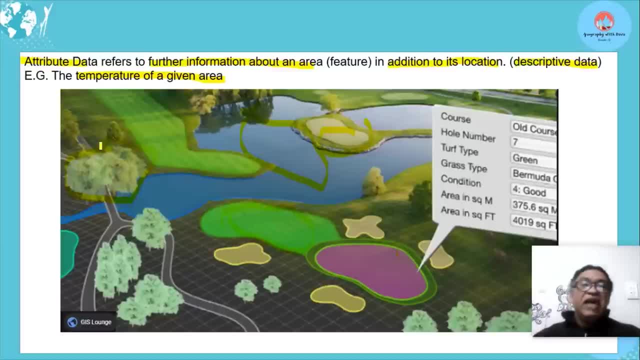 minutes, whatever south and east. and what else do we look at it? what describes it? okay, all the different features. that is actually had to be beta. it is descriptive time of data- all right. or it gives you further information about an area in addition to its location- good definition. but if you want it just simply in two words, it actually is descriptive. 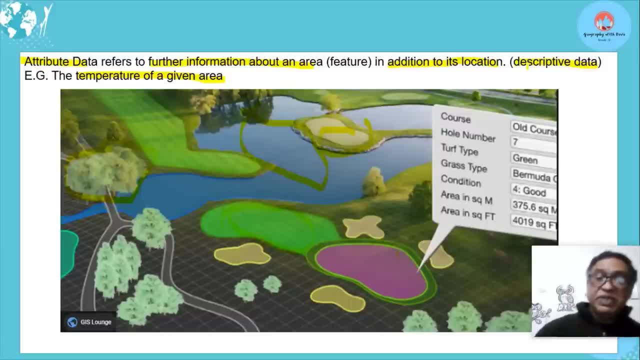 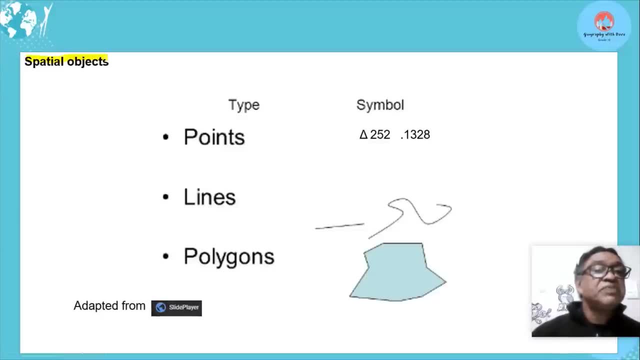 data about a feature. okay, right, let's go on spatial objects. you've done this before. all right, i know for many years, from grade 10 onwards, you've done this. points which can be your trig beacon, your sport height, the symbols, like church, whatever. those are your points. 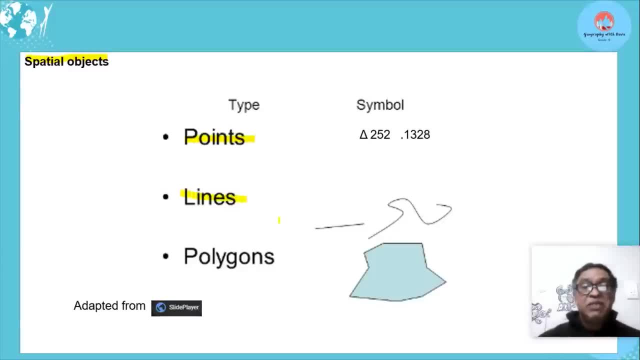 then you've got lines, which can be your railway line, your rivers- all right, roads, those are line features. and then you've got polygons- same like maths. you've got polygons- same like maths, all right, your features. that irregular and enclosed- okay, like the dam, yeah, built up area. 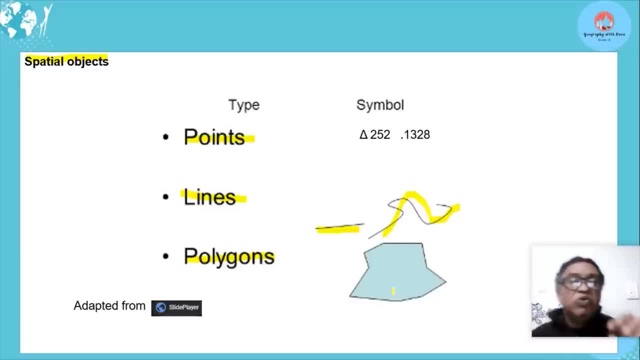 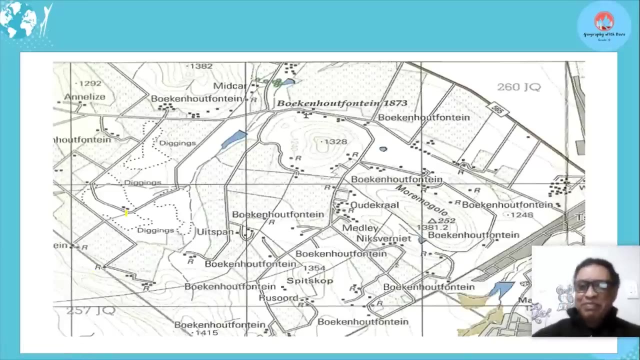 cultivated land. all right, those are polygons and these are the three spatial objects that you have dealt with before. but we're actually going through all, we're not taking any chances. now, where is spatial objects used? it's used on a map. all right, on a topographic map. you see here, you'll see all. 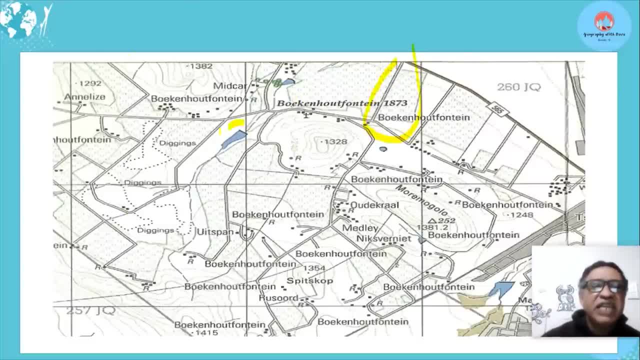 these secondary roads here? all right, there's a dam here. the road would be a line. the dam will be a polygon. you'll see cultivated land here. that's your polygon, all right, you'll see the reservoir. that's your point. this farmstead is a point, can you see it? all right, there's your spot height here. 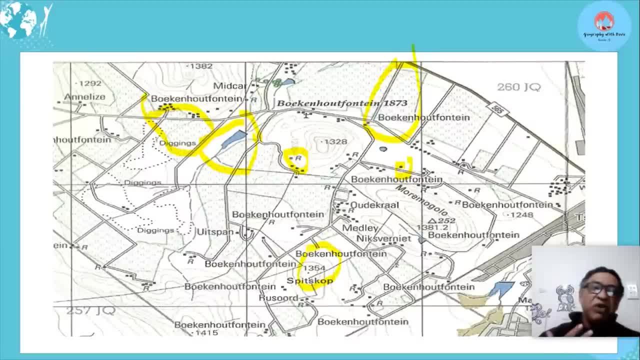 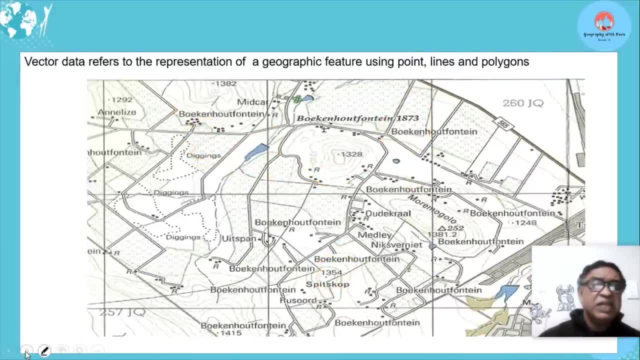 which is your point. there's a dot there, so we know polygon line point. all right, that is your spatial objects. can you see? it's simple, learners. vector data refers to representation of a geographic feature using points, lines and polygons. so vector data is not an image, it's a representation. vector data. 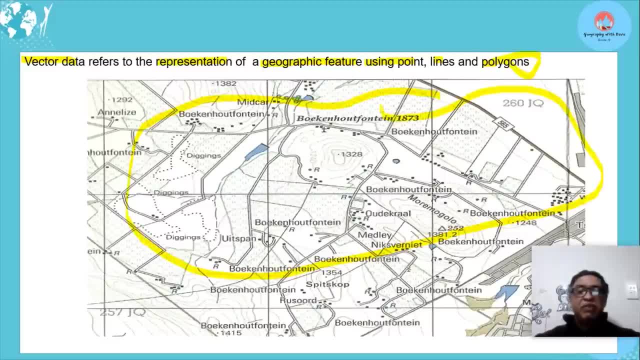 beautiful. you'll always be using. it is your topographic map. can you see, as i showed you before, there's polygons used here, like your dam, your cultivated land. there's lines like your roads, there's dots points, uh, like your, uh, your reservoir. so all is being used here, so you use your polygons. 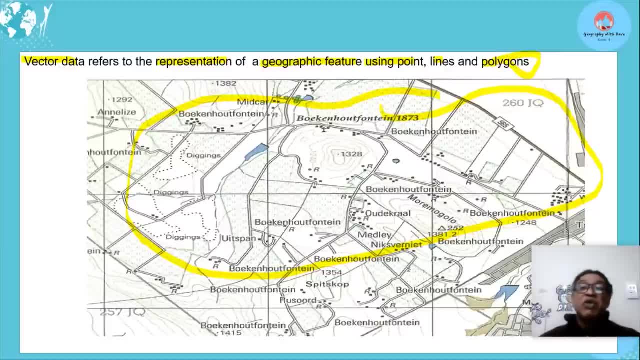 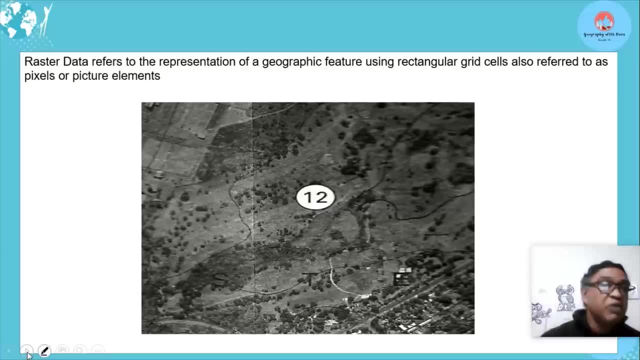 is not everything needs to be used at one time, all right. but as long as you got these things is vector data, topographic map. remember that. you will not forget it then, if you remember that topographic map, vector data, raster data, is a represented representation of a geographic feature using 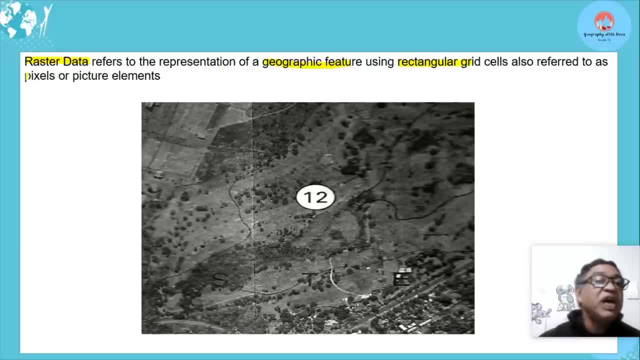 rectangular grid cells, also referred to as pixels or picture elements. beautiful is your topographic, not your topographic. my, do apologize, is your auto photo map? all right, it's an image. that is why it's using pixels. it's using gr, also known as grid cells. all right, but the best is the word pixels. 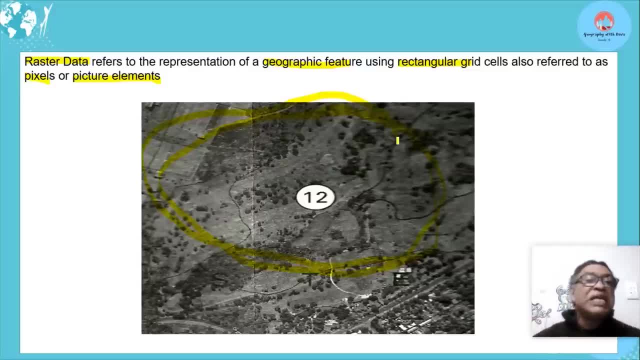 okay, and therefore it's is becomes an image or a picture. that's your raster data. so vector data is representation points, not lines, polygons. all right, it's like a topographic map. raster data is a picture. okay, like your auto photo map. all right, i'm messing up this one. let me go on then. data layering. 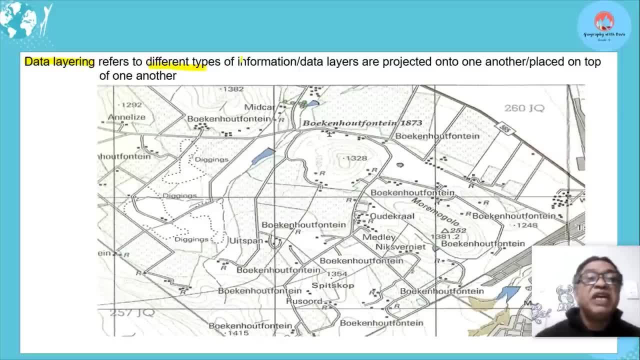 here we put the different types of information or data layers up projected onto one another, or we can say it's placed on top of what another. so we take different data layers. like: one data layer could be drainage, all your rivers, etc. another data layer could be infrastructure- your roads and things, or transport- all right. another day data layer could be: 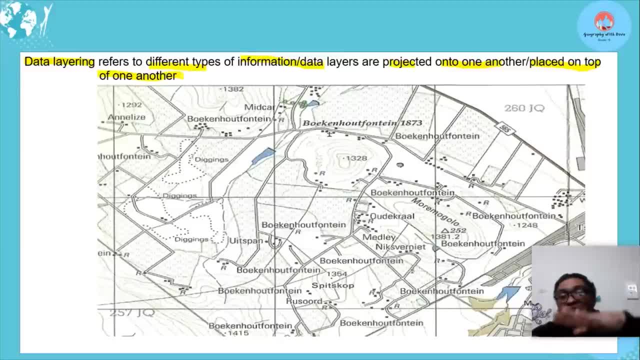 vegetation. and you take all those data layers and put it together, but you put them on top of one and other. all right, data layers are projected onto one another, or we can say it's placed on top of one another. all right, don't forget to put them together. and what do you have? 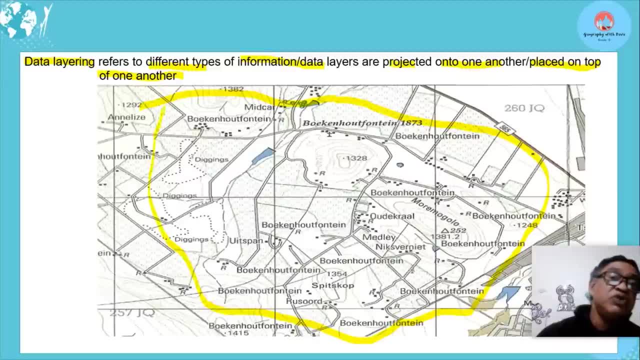 your best example of data layering that you will be using in even in the final exam is your topographic map. can you see different layers? there's a reverse drainage, there's the cultivated lands, agriculture. can you see your road networks, your transport, or put on top of one another in order to create a topographic map? this is data layering. to 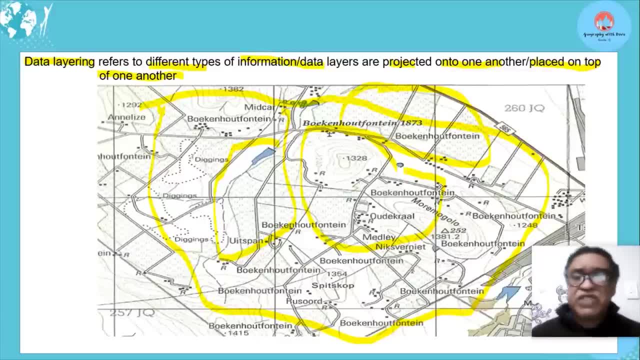 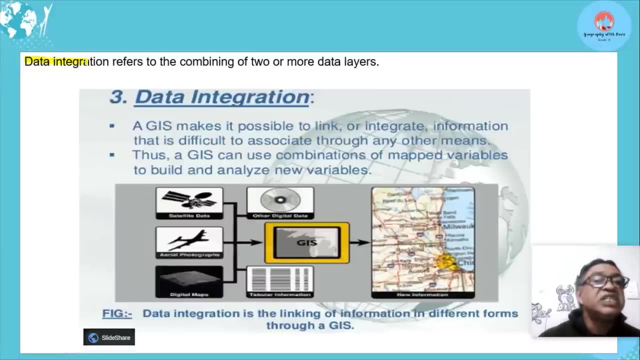 don't go too far. i know there'll be a lot of examples, a lot of scientific examples. you stick simply. you know, players on top of one another is a topographic map. okay, let's go on then. data integration refers to the combining of two or more data layers. now, 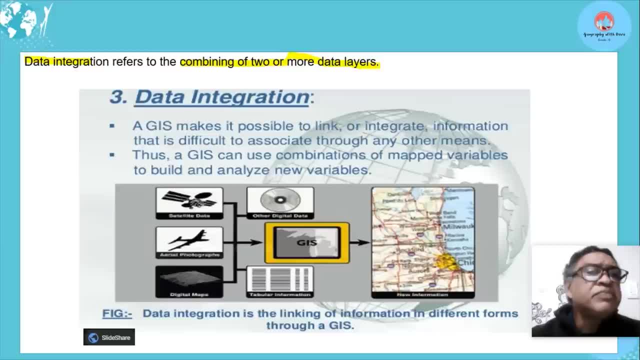 data layering, data integration. you may say: what isn't that combining? what's the difference? remember, in data layering, you're putting layers on top of one another, all right. in data integration, yes, you will put players on top of one another, but it doesn't necessarily have to be on top of. 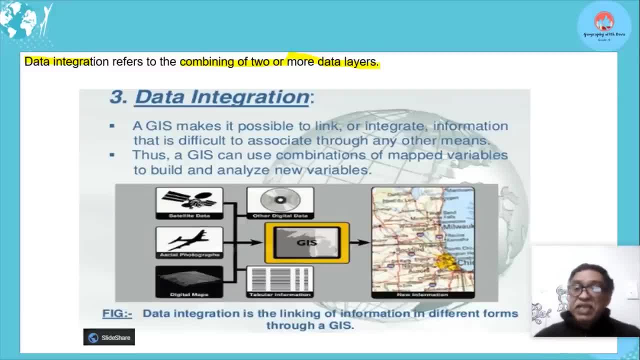 one another. it can mean different things. you can take figures you understand and bring them together and work out where's the highest crime in an area. okay, how many robberies are here, how many robberies are there? you can bring statistics like that and put it together. it's not putting it on top of one another. so data integration or data. 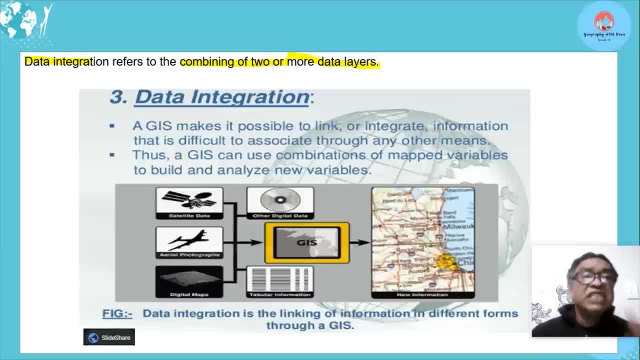 layering is one type of data integration. okay, and it gives you an example. here you get satellite data, data from digital- all right. other from this that you're going to use, that you obtain from people- all right. you're going to use tables- all right, digital maps. and eventually you're going to take all this, put them together and 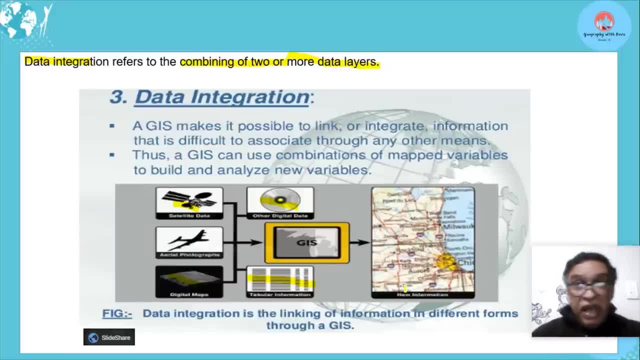 make this map or you're going to get figures: how much hijacks were there in all the areas hijacking, how many robberies were there, how many house breaks they were? you're going to put all the data to determine which is the safest area. that's also data integration, not putting it onto one, and 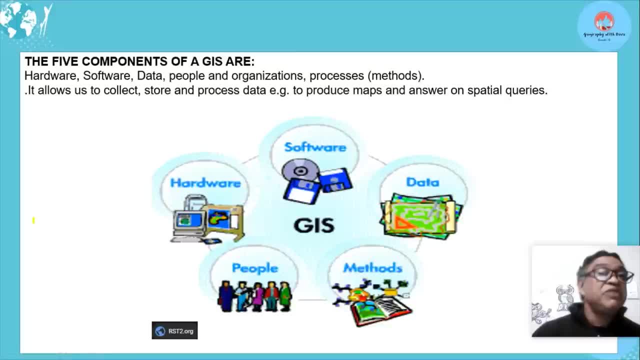 other or top of one another. okay, you understand the difference between those two. then the five components. i know you say, oh, not again. all right, but it's part of our matrix curriculum. let's just go over it a bit. you know, it's hardware, it's software. 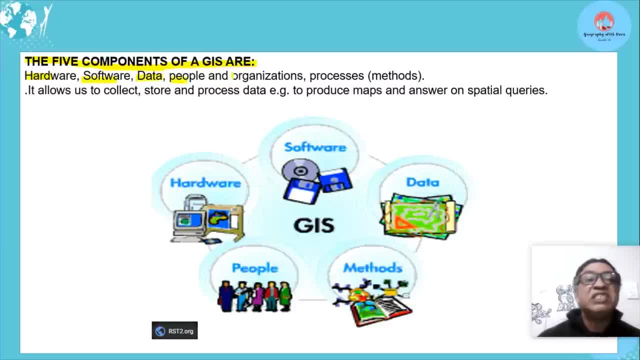 it's data, it's people, it's organizations with an s: okay, it's a, that's a process and methods- okay. so let's look here: if we don't have the hardware, the computer, etc. we can't do gis. okay. then if we don't have the software, like the art program, etc. 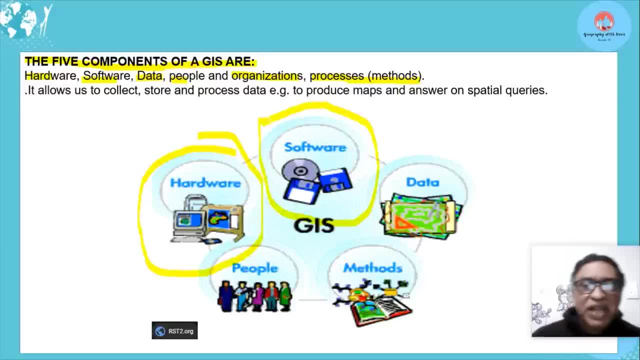 a computer is not just going to get it like that. we need software, all right to be used with the hardware. okay then the data, the information that we're going to use, like those statistics i told you. we need to get information about where's the crime, how much hijacking was there. if you don't, 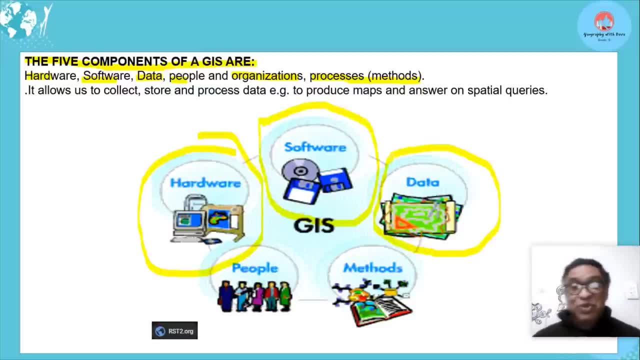 have the information, you're not going to be able to do gis also. then you need the methods by a data layering, data integration, whatever. okay, all that, and eventually, if you don't have people to do it, who's going to do it? i don't know the future. maybe computers will do all these. 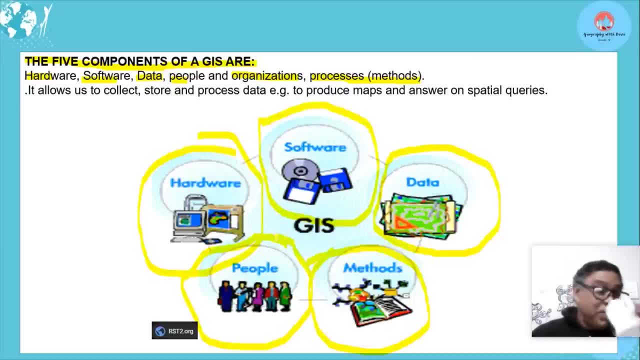 things i don't know, but now even computers have to be designed by man, okay. so, oh, by humankind. i do apologize, i'm being chauvinist there. it's not just man, it's humankind, all right. so all these things work together to create the gis, all right, that's why it's five. 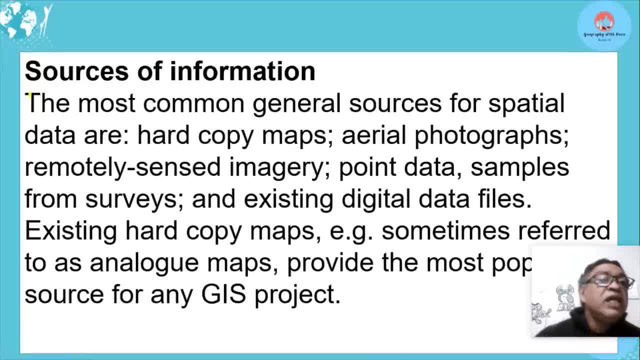 important components. then in your stuff you will see the word sources of information and you say: what is this? it's just basically telling you where we get sources of information from for gis, so do not get confused. i know even some of the learners that i teach sources of. 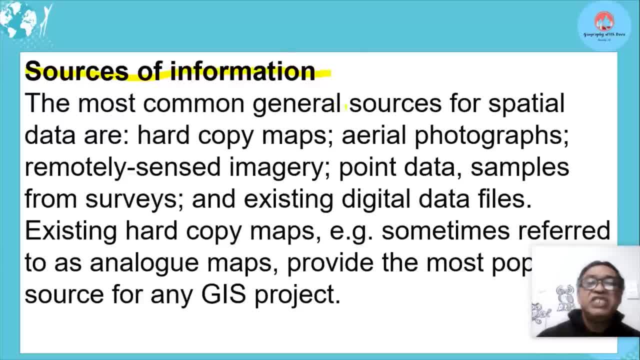 information. i don't know what are they? okay, do you look at this? they are general sources for spatial data and that's what we're dealing with: spatial data, location and descriptions of the locations, etc. hard copy maps that you have can be used, aerial photographs that you use where. 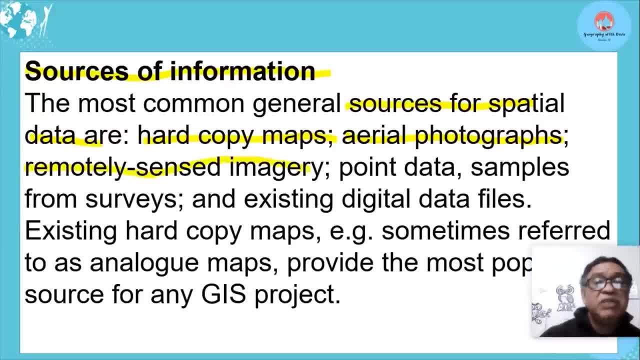 photographs turned into your auto photo maps, remote sensing imagery that you get from the computers. point data- all right, samples from surveys, pre-existing digital files. can you see information that exists? all right, samples that somebody took as a survey. you want to use that to determine? okay, existing maps. sometimes refers to an analog maps. okay, uh, most popular. 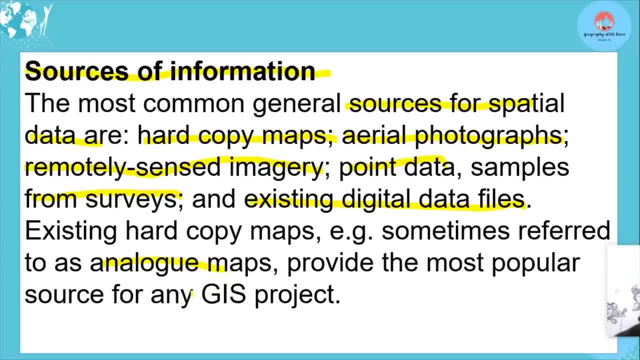 gis project. all right, these maps that you use. so it's where we get our information- can be from research, can be from, uh, other digital information that's already been stored. whatever that's the sources and we get a question based on this: learners look at which sources they talking. 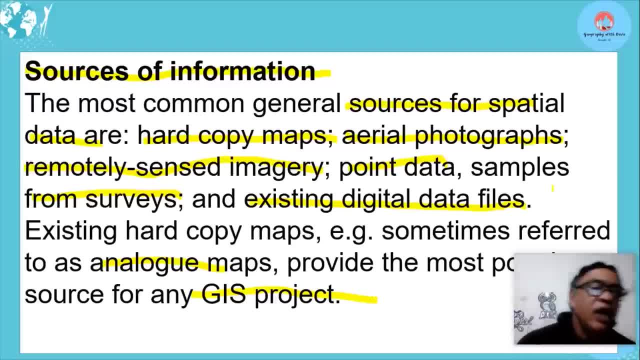 about there. okay, this source was taken from, uh, from a survey done, you understand, on an area. so you, if they ask you the type of source of information, then you talk about surveys. okay, and there we go again. i must mix it up, okay, apologies for that. learners, let's go next. 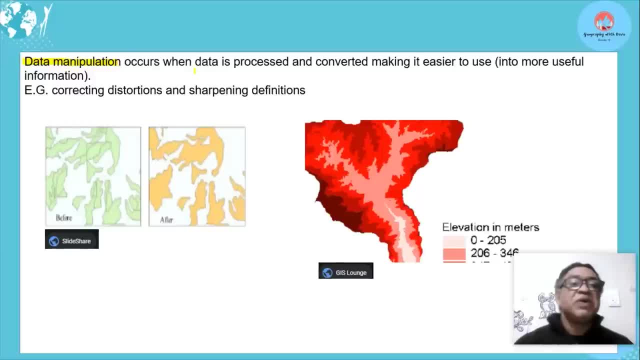 one, data manipulation. okay, here data is processed or converted, making it easier to use, or, we can say, more useful information. okay, that's your definition: easier to use, it's processed, it's converted, it's changed, so it makes it easier to use. all right, let's take this. 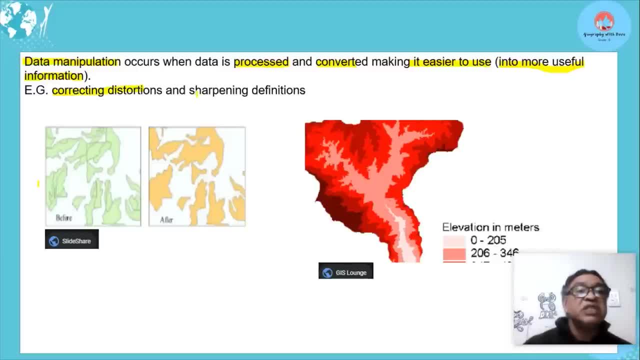 we talk about, example here, correcting distortions, sharpening definitions of the picture. all right, this had many lines. we don't really clearly see the shape, the lines crossing, etc. all right, what we've done here. we want to see the outlines. we've removed all that and we just have a map. 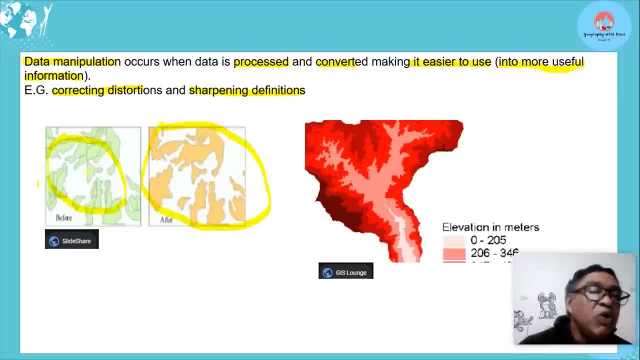 and now it's clearly seeing where they're meeting. yeah, we don't know. you're right, it looks as if they're meeting totally there. uh, lines running across. so we made the. we corrected the distortions in this. all right, now look at this. okay, we made it more useful. we. 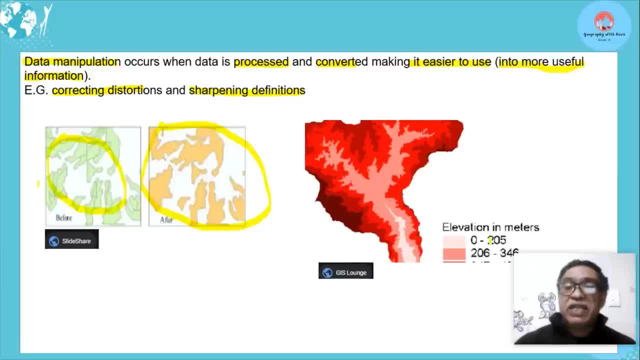 use different colors, etc. okay, to show that this lighter color is 300 uh 206 to 346 meters. okay, the very light color is zero to 205 meters in terms of elevation. can you see what we're doing? manipulating the data to see the imagery. okay, so this is what happens here. all right, proceed to. 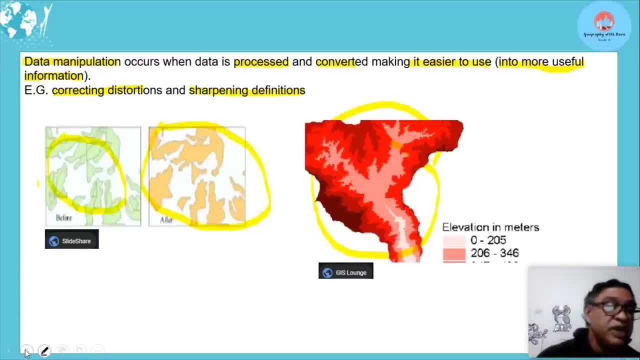 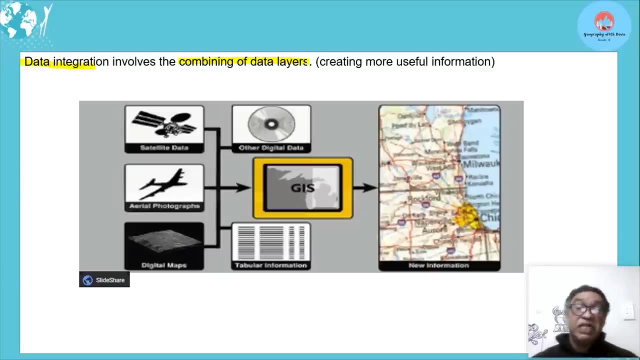 convert. making it easier to use. okay, remember, there will be slightly differences if you use different words. long as you mean the same thing is fine. all these are concepts. data integration involves combining layers of information. i think i've repeated this. okay, creating and making it more useful. there's another definition: combining layers or data layers, making information more useful, okay. 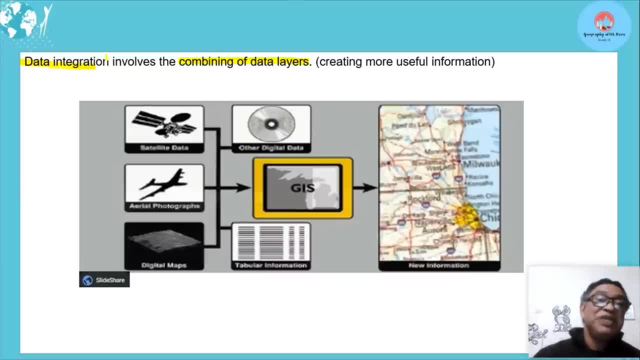 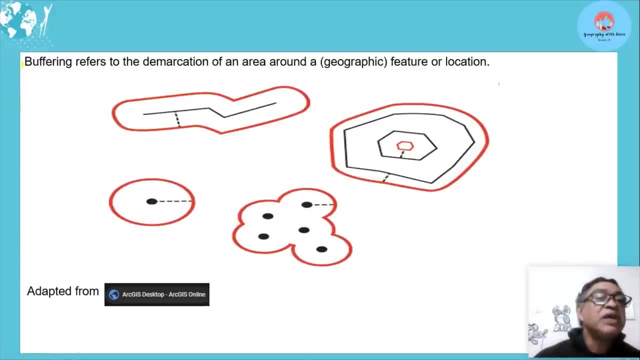 but i did cover this before. but i i think the slide is not wasted because we've got another simple definition. okay, let's look at the next one: buffering. now watch out, learners, if you want to get your full one mark, i know somebody's one mark. why am i having to work so much? 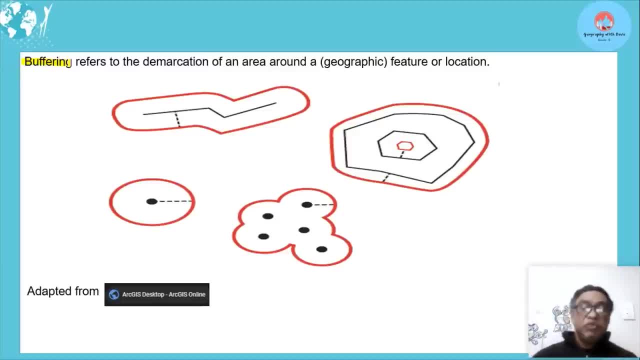 always even a definition for one mark. you must give the full definition. many learners write it's a demarcation of an area. it's too vague: around what? what demarcation okay? so you have to be specific. it's a demarcation of an area around a feature, or you can write location. 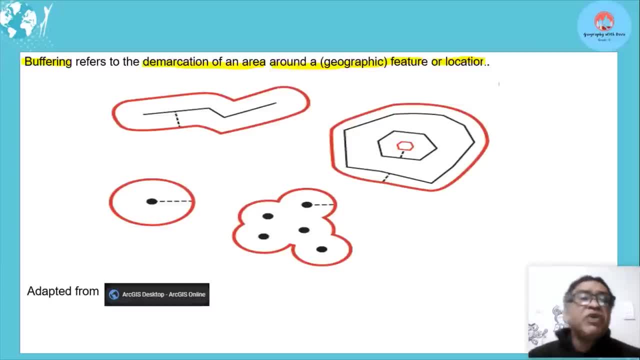 now put geographic in in brackets. that's correct. but if you wrote it's a demarcation of an area around a feature, you got your mark. okay, don't write around an object, please. an object is my coffee mug here. all right, that's an object. you must say feature. 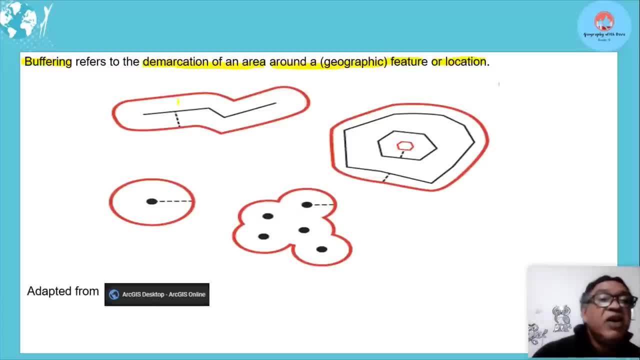 or you can say location: look at this. all right, this is a road or a river. so buffering around a line- all right, maybe this was a river and it could flood. therefore, we buffered and said: no development here. this is a buffering around a point. okay, where you actually look at, maybe it's. 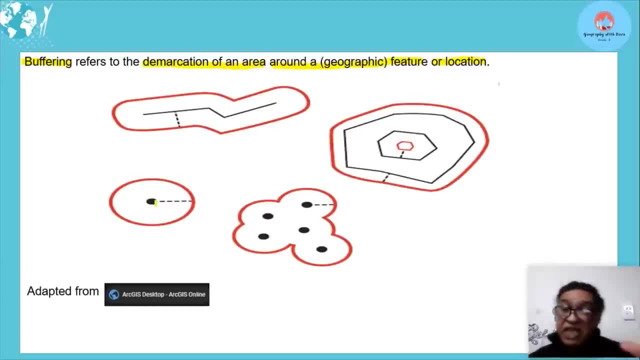 a nature reserve, we don't know, all right, whatever, but nature is a bigger than that. uh, maybe it's school, okay, and we want to know from which area do we have the feeder zone to come to the school? you know feeder areas? all right, this is buffering around a polygon which could be your nature. 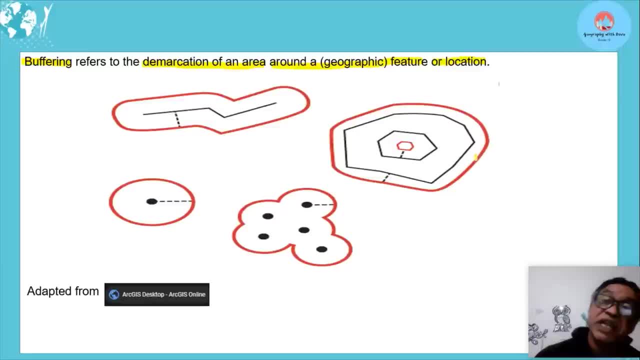 reserve. now you buffered and said: no development around this nature reserve, all right, so we stop development here, we keep this for conservation. then there's various points where you can have buffering. so it's demarcating an area for various things: to stop flooding, to stop this, to stop that. 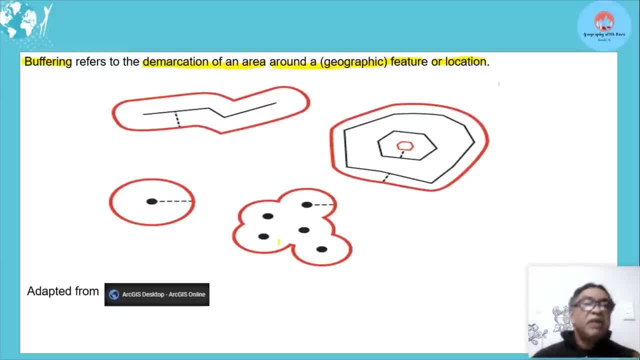 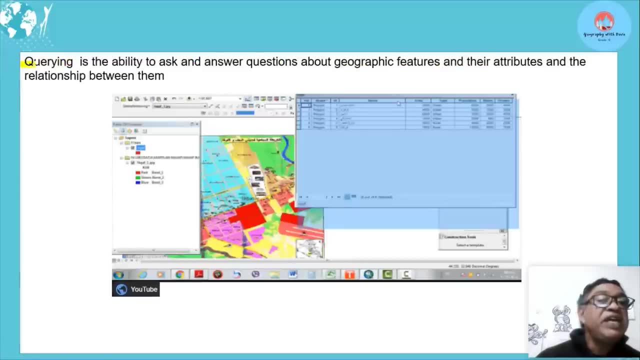 you understand to stop urban development, okay, but it's demarcation of an area, it's a demarcation of of an area around a feature or location. then query: what is that? of course you queries, ask, okay. ability to ask and answer questions about geographic features and the attributes. 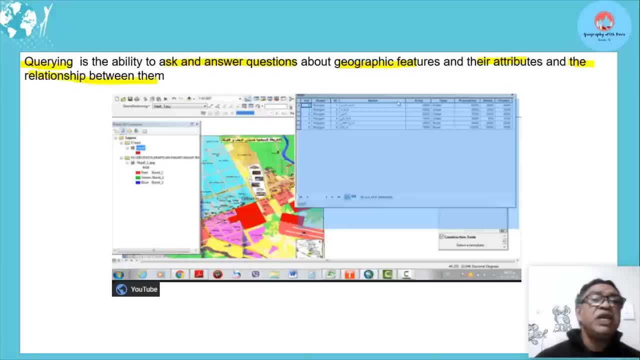 and the relationship between them. quite a long one. you can ask questions about geographic features, okay. attributes referring to their descriptions, about the data and how they related. okay, now let's look at this. i'm just going to make a hypothetical system here. all right, i want to know, using my gis. 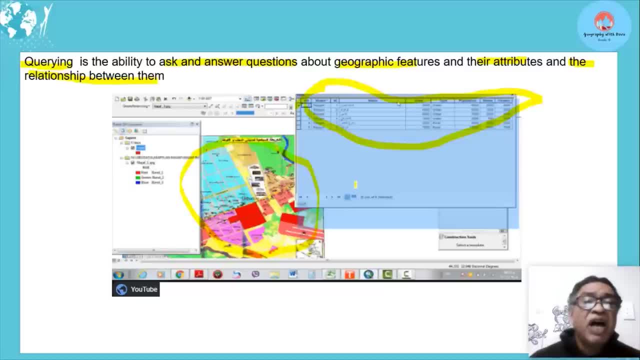 all the data that i have, etc. i want to ask: which area is a crime hotspot? okay, so i'm going to look at the features of the area and their attributes. oh, there's this area here, this area here. whoa, there's policing here and hardly any crime here. hardly any crime here. because my query 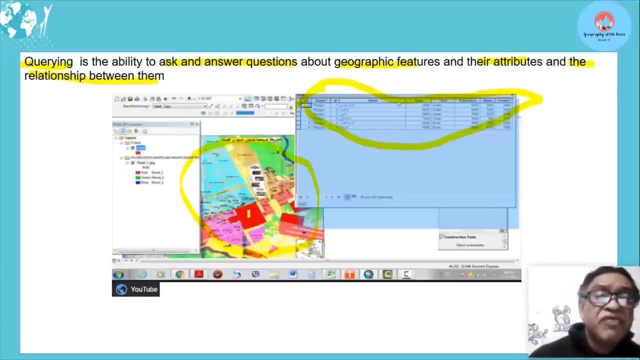 is crime. where is the crime the highest? and suddenly i find here, whoa, lots of murders and lots of break-ins, lots of this. i'm sorry i'm using the crime thing as an example, but i all the time, but i used it before. oh so this is a hot spot. i can mark that off. 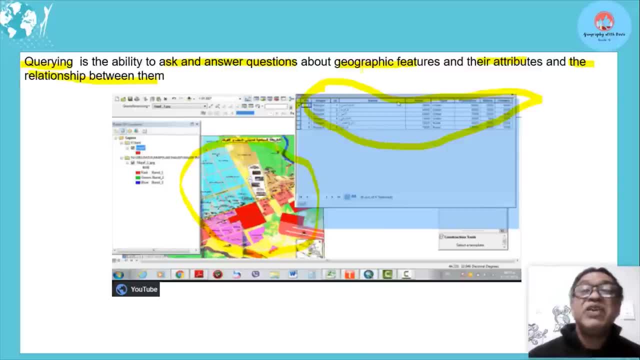 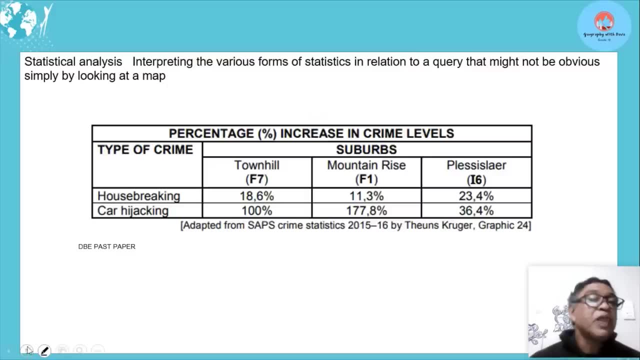 but i'll get back to you in just a second. so this is what you can improve on, okay. what are these categories? this, this is what you can improve on. okay, so now i have three categories in which my query is based on first three, my query- and then looking at all the features and 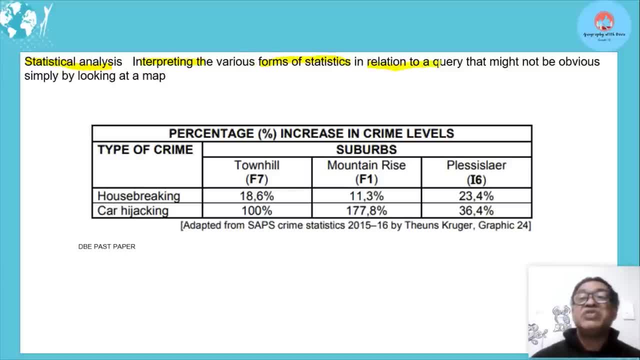 descriptions in terms of getting my answer. okay, statistical analysis is interpreting various forms of statistics, okay, so here it involves figures, etc. okay, so let's look at it. my query here is: i've got different suburbs, all right. i've got town hill. i've got mountain rise, i've got. 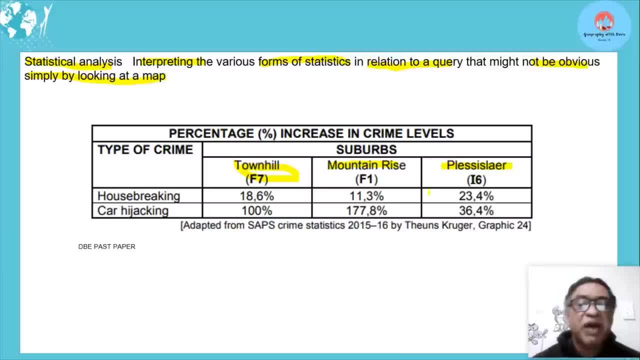 precisla. all right, i hope i'm pronouncing that correct, but my apologies. and i'm looking at two things- car hijacking and house breaking, all right, and i want to see which one is having a higher crime rate. okay, if i look at a topographic map, he's not going to give me that, so therefore i 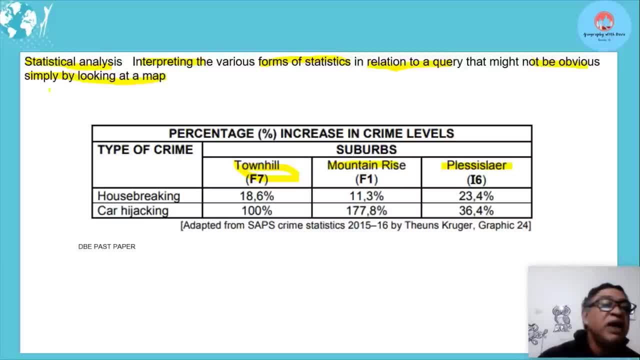 look at statistics. that's why it's not obvious by looking at a map. okay, i have to look at statistics. can you see statistical analysis and then analyze it? whoa, yeah, it's 18 percent. in town hill. 11.3 percent, all right. yeah, 23.4 percent, okay for that place, all right. 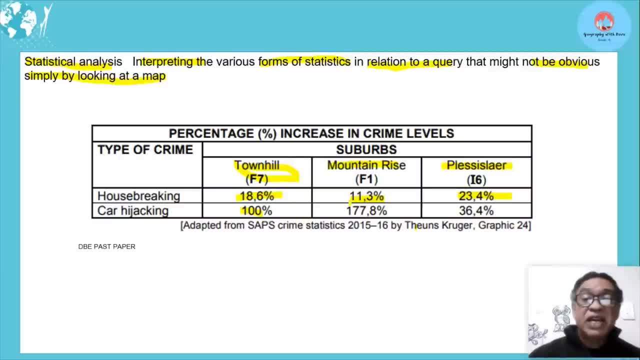 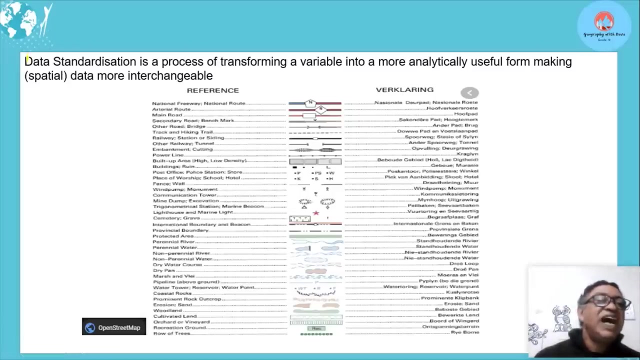 car hijackings. can you see 100, 177.8, okay, 36. i can work out which place has a higher, which place is lower and then determine where my crime rate is high or low. can you see it using figures, statistical analysis- nothing is difficult in gis, then data standardization. 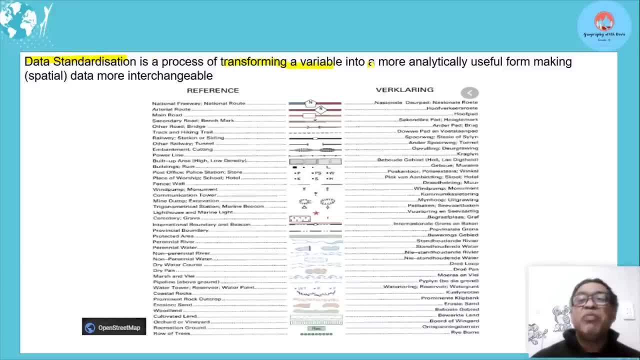 transforming a variable into a more analytical and useful form: okay. making data more interchangeable: lots of heavy words there. let's make sense of this. take maps in south africa. let's see. each map made different symbols. some maps, all right for cultivated land. they had circles, okay. some maps had little lines like that. some maps had crosses- okay. 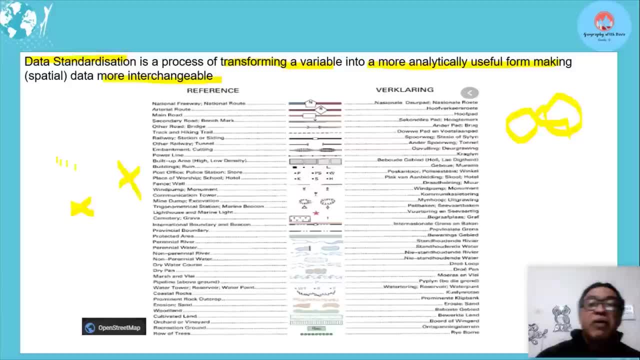 then for each map you'll have to have own reference. all right, but what if you? this is the most correct one, okay, but what happens here? if you decided to create a reference, all right, and all south african maps will have little green lines for cultivated lands. national roads will be your red and blue, all right, uh, railway or lines and station will have that. 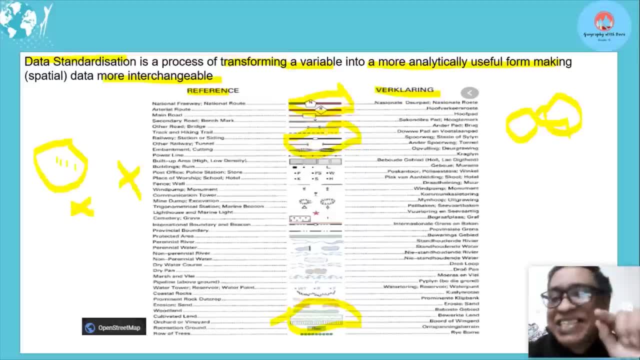 symbol. what have you done? you have standardized the data. i don't need a topographic map of south africa, i don't even need to have the reference there. if lenders know, if people know the reference, all right. they can just look and say: those little green lines is cultivated land, all right. 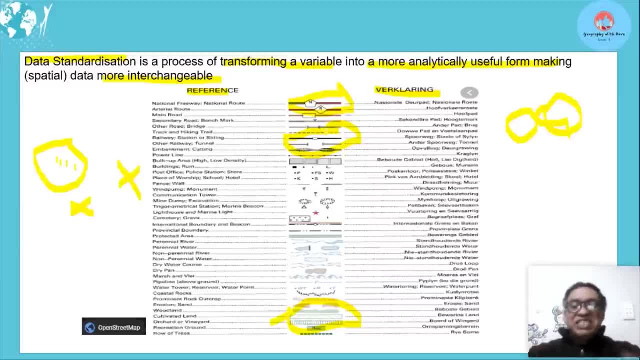 a thick red line is your national road. this is data standardization. your maps have data standardization. don't get into any other complex things, so we're taking a variable. this could be a variable if we use different symbols and into more analytic and useful. so we took these variables where each one may have different symbols for cultivated lands. 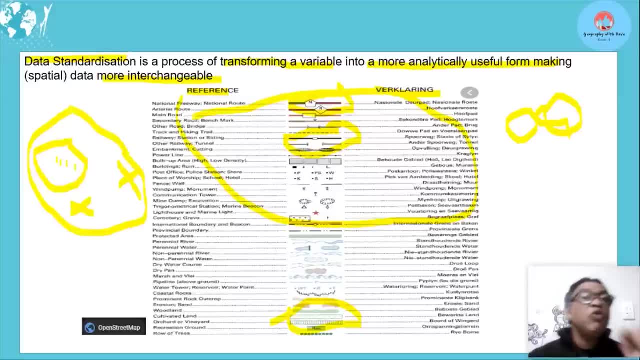 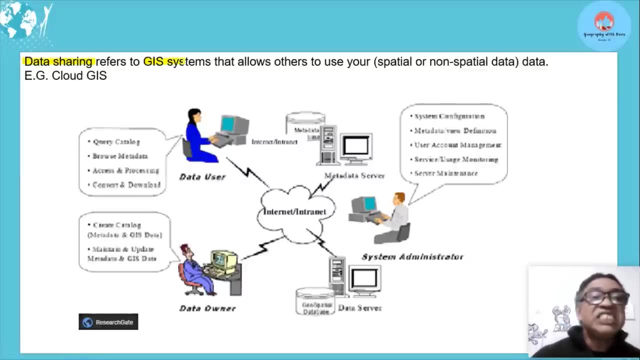 and we made it one which becomes more useful and more interchangeable. you understand it can be shared. anything okay. data standardization, your topographic map data sharing- okay. a GIS system that allows others to use your data. I said spatial or non-facial, but if you said allows others to use your data, all right. 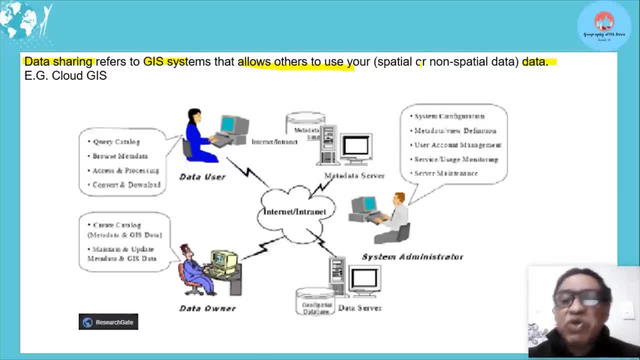 I think maybe you should mention your spatial or non-spatial because it could be others to use your data. means you got data on your phone- 20 megabytes, you understand- and somebody else uses it. okay, so allows somebody else to use your spatial or non-spatial data. now cloud it gets started. people can use it. you. 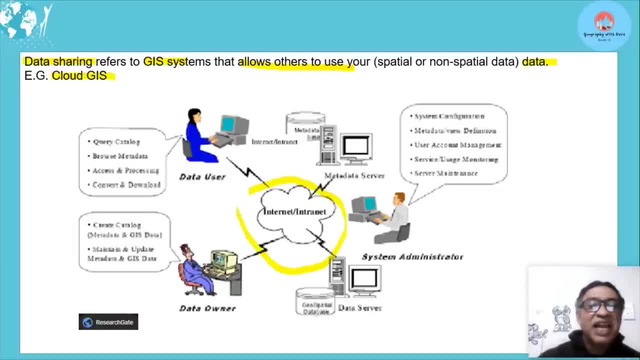 understand the internet, okay, allows you to share information. at this stage, we find when, when people are not able to go to school due to various things like covered, etc. over 90- this information is shared through zoom, through whatsapp, isn't it? it allows systems that allow you to share. 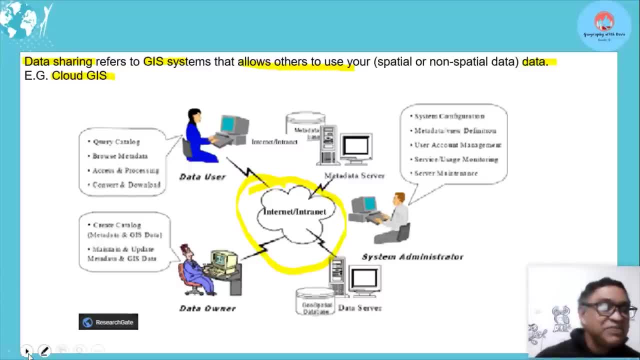 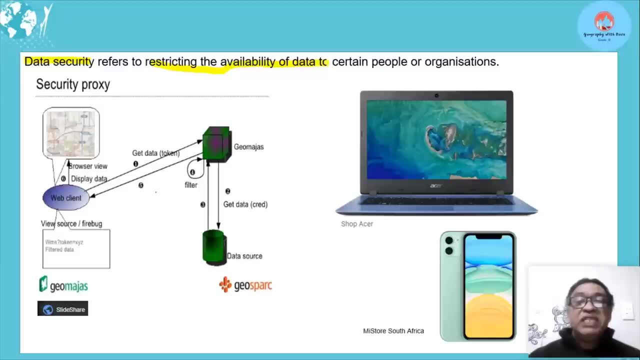 data, okay, data sharing. data security refers to restricting the availability of data to certain people or organizations. like here we've got a very difficult one. we look at how this data gets sourced. it goes to a web client. they can only get the information. all right, let's take something simple. let's leave all that. 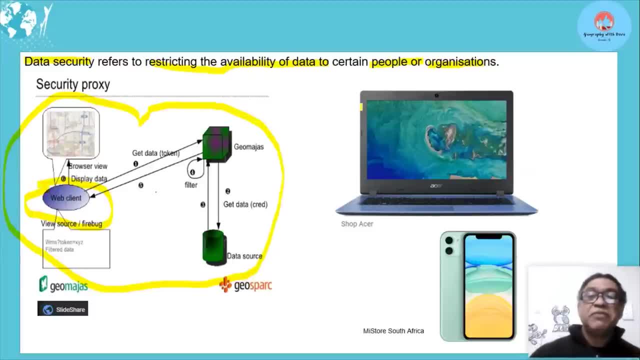 all right, let's take this computer. okay, you may have data in here. all right, you may give people access. I'm just using not totally the best example, but it makes you understand it better. all right, you may allow people to open that up, because the data has a code on it. now that computer has a code on it, you open. 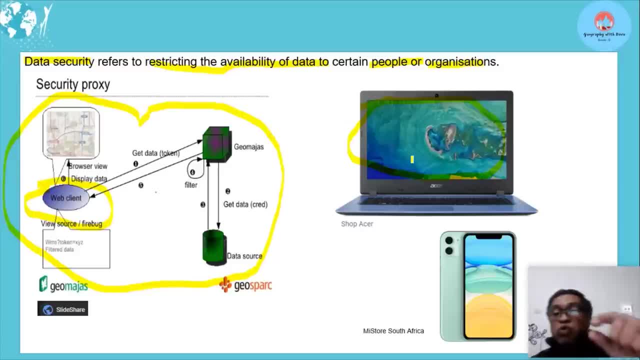 it up and you share, or you may put codes on different articles- that only some, and send people the code from your computer to say: this is the code, you open it. if it's confidential information, all right, so they'll get the thing, the information, but they won't be able to open it if you don't give them the code. that's data. 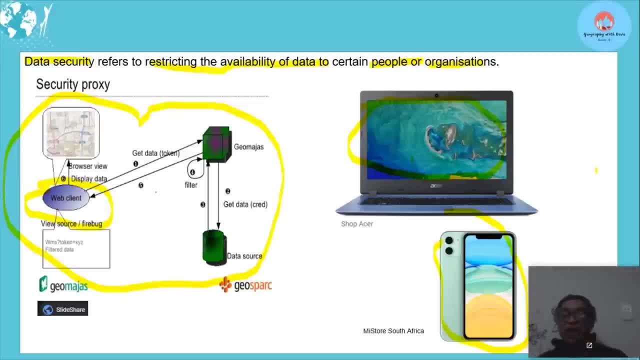 security your cell phone. you know some of you zip around with all the fingers, or you type out something, or you put your finger somewhere, or you put your face and that's what it can open. all right, so certain people can open it. all right. so data security and must know your parents can open it. don't think they don't know. 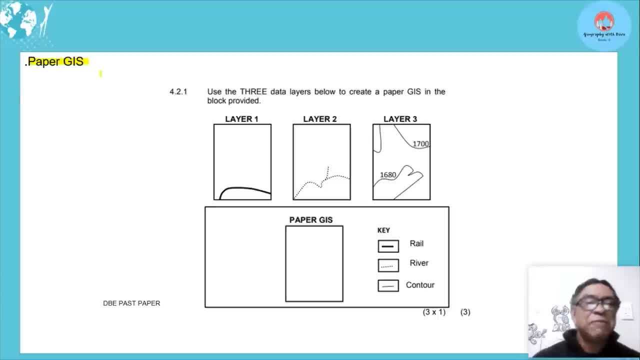 GIS- all right, paper GIS. people get so confused with this. learners, it's something simple. I'm gonna just use this: all right. where in this past paper, what happened was they said: use the three data layers below. it was taken from the map: the three blocks- all right, and make a. 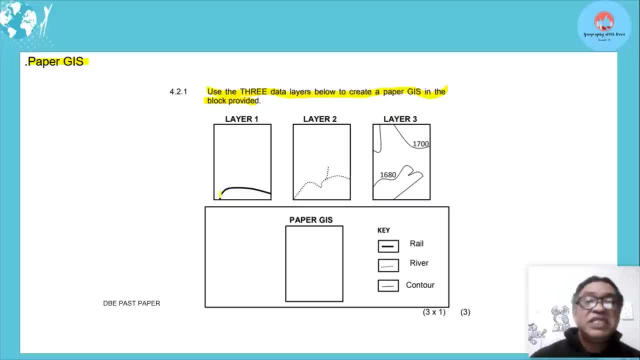 paper, GIS, all right. so this represented your rail, this represented your River and this represented the contour lines. all right, so what you have to do, you have to take all of this and put it together. yeah, it was here to determine where's the best place to put a factory, so obviously, rail. 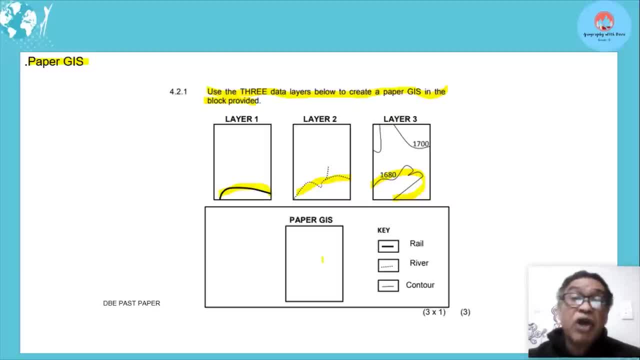 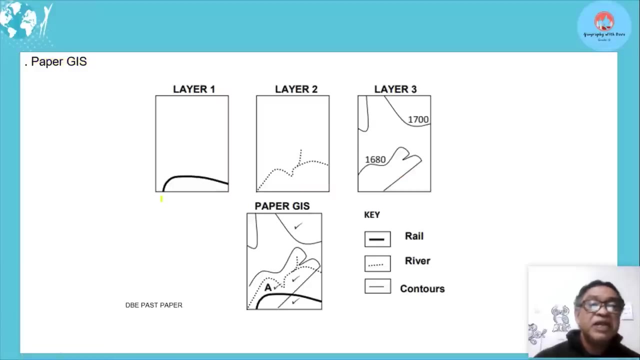 for Transport River for water supply, uh, contours in terms of Flatland, and you have to put all that together to create a paper GIS. so the word seems more complicated than anything else. now look what you have to do for this question. there's this one here, all right, the rain. you put it exactly where. 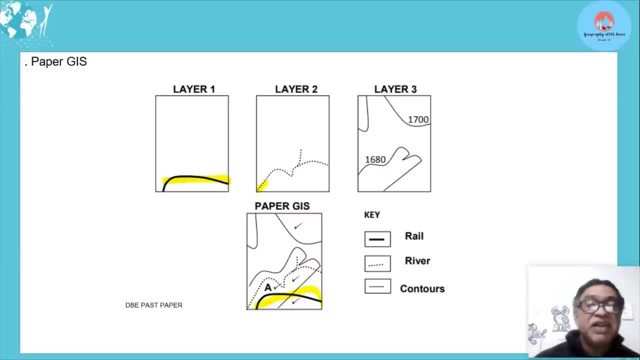 it's supposed to be there. you just copied it from there- the river. can you see that? you took it and put it here exactly where it was, the contour lines, exactly where it was. and now you see, oh, places like a, it's near the river, it's near the railway line and it's generally Flatland good place to put my. 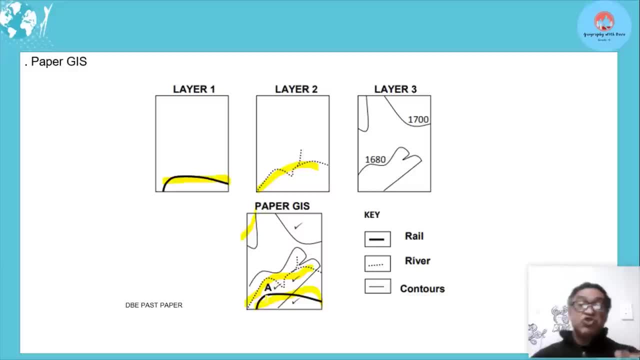 factory. so you actually did a paper GIS to sort out the query. your query was: where's the best place to put your factory? yeah, it was near the water, near the rail, near the river. learners, GIS is simple. you just need to consider it yourself. all right, people get confused with buffering. I say we do buffering. 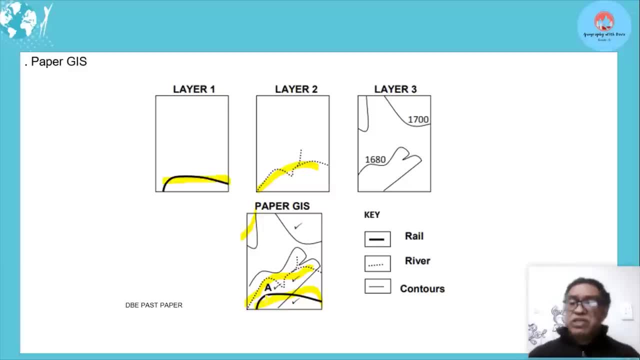 we determine how far from the school can learners come to that school. isn't that buffering your feeder area? you understand, okay, you look at various things. so GIS is a daily use. through your computers, through your cell phones, you're always getting data. you want to do a project?